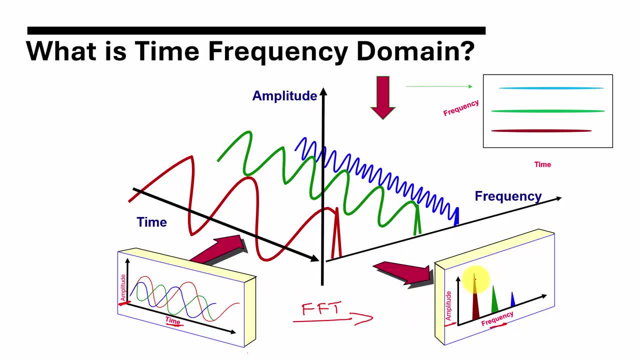 based on the pattern of the signals, we can identify the faults. Now coming to time, frequency domain analysis. this time frequency domain has time as the x axis and frequency as the y axis, Based on various transform. I will come to that later. So this time frequency domain. 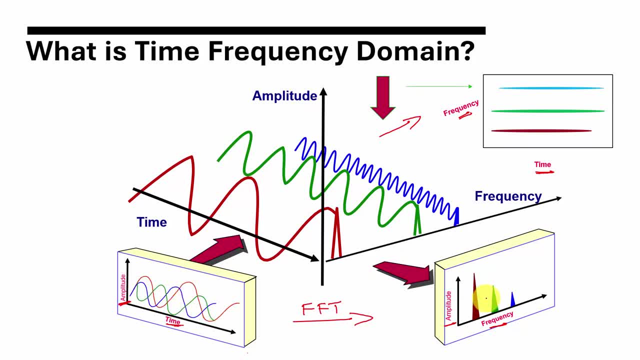 analysis has the information of both time domain and frequency domain analysis. So the analysis of non stationary and non linear signals will be carried out very easily with the help of time frequency domain analysis. So here you can see that there are three signals. are there In time domain analysis? we cannot split the three signals individually, In case 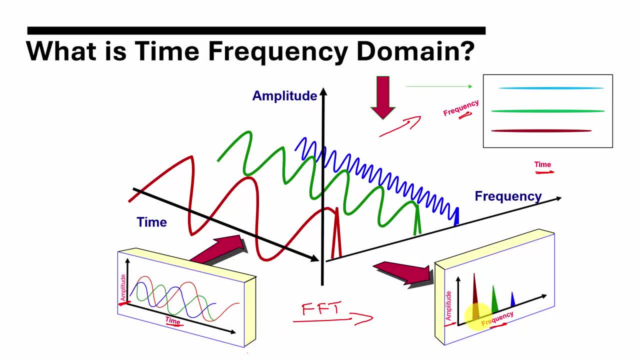 of frequency domain analysis. we can split the three signals individually. So if you are, apply x lazily and x into random line, you can go and you can interpolate this in: at what frequency, how much is the amplitude. that is what the information we can get it. 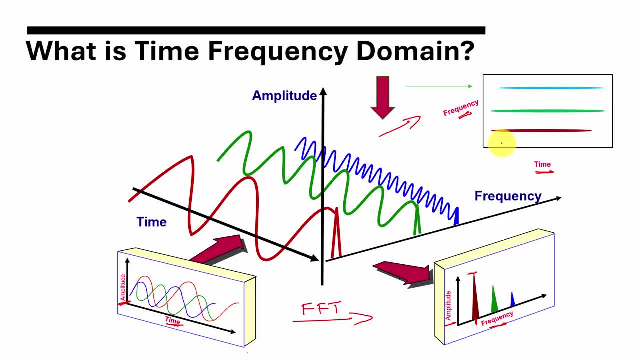 from the frequency domain. In case of time frequency domain analysis, we can identify at what time, at what frequency the energy concentration occurs. So we can get the information of both the time as well as the frequency. So this will be very easy for fault identification. 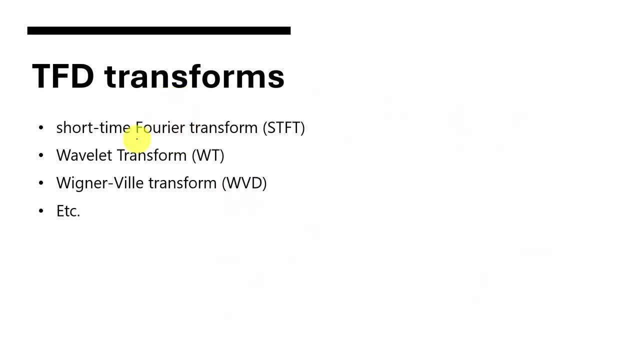 There are many time frequency domain transforms are available. The most common types are short time Fourier transform, then wavelet transform, then Wigner-Weil transform. Nowadays people are using CWT, continuous wavelet transform, then Q-transforms. there are plenty. 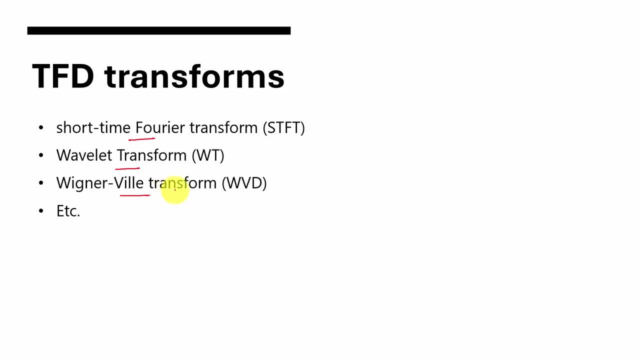 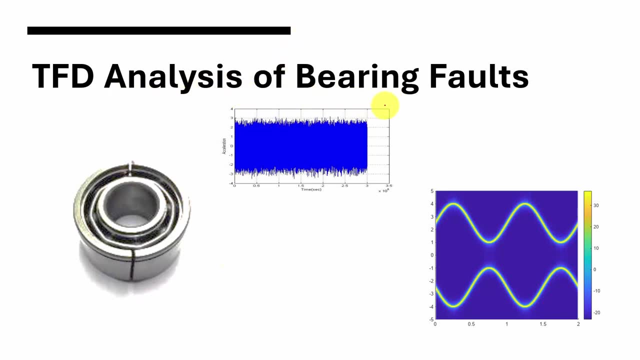 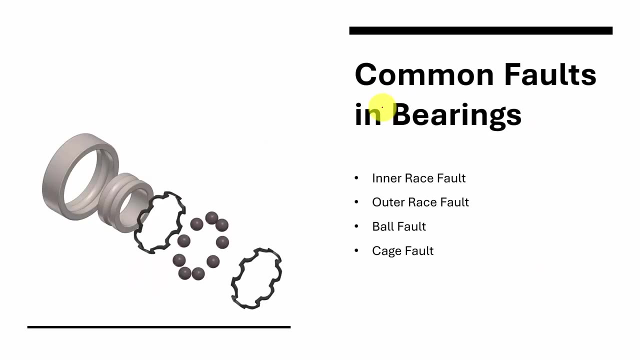 of transforms are available, So each transform will increase the effectiveness of the fault identification. So, first of all, time frequency domain analysis of bearing faults, So how the faults in a bearing can be identified Using time frequency domain analysis. In general, the bearings are subjected to these four types of faults: 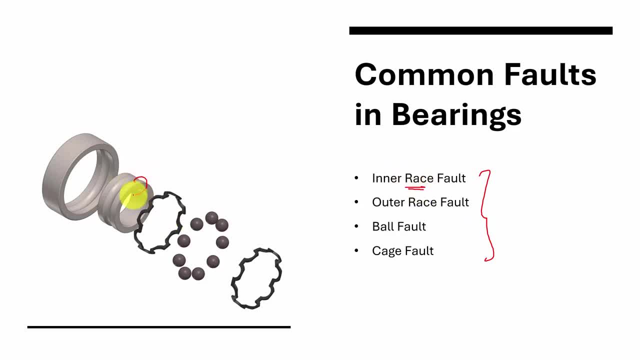 So one is inner race fault, that is fault at the inner race. You will have a crack or maybe a pit hole in the inner race. Then second one is outer race fault. Fault in the outer race, Then ball fault, So there may be a defect in the ball. 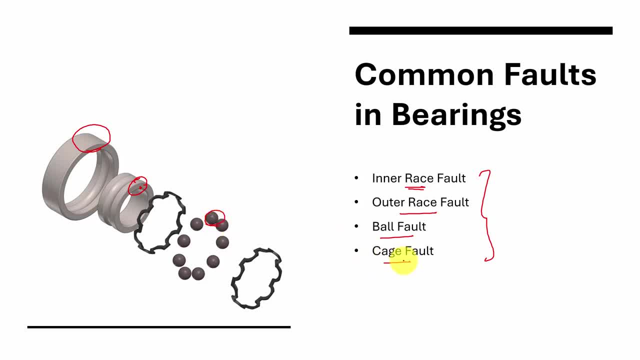 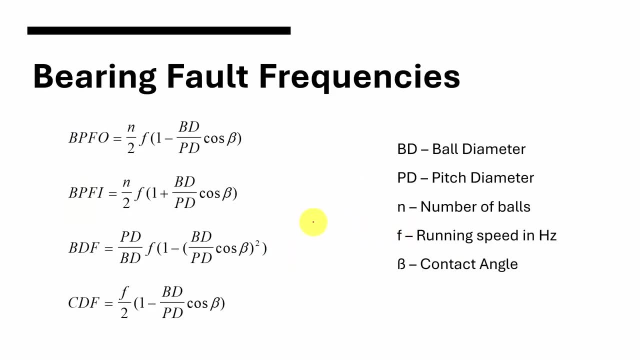 Maybe a worn out ball will be there. Then the last one is gauge defect, So fault in the gauge. So these four are the common faults in the bearings. So before going for fault identification of any components, first we must identify the fault frequencies. 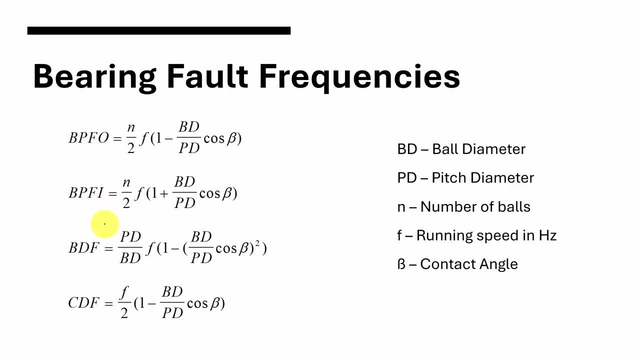 In case of bearing, as I said earlier, there will be four faults. So there will be four fault frequencies. So BPFO is ball pass frequency- outer race, PPFI is ball pass frequency- inner race, then ball defect frequency and gauge defect frequency. So these are the equations for calculating the fault frequencies. 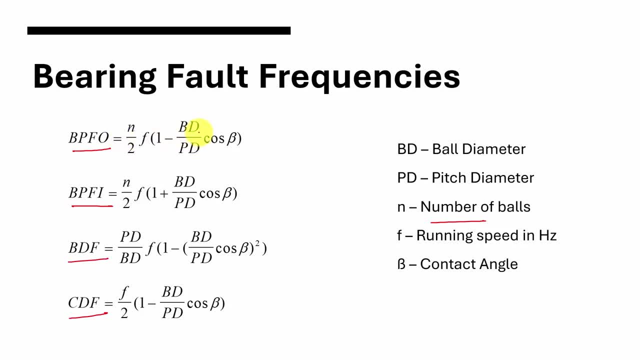 So here, N is the number of balls and BD is the ball diameter, PD is the pitch diameter and beta is the contact angle of the bearing and F is the running speed in heads. So now, before going to the fault identification, you can get the specifications of the bearings. 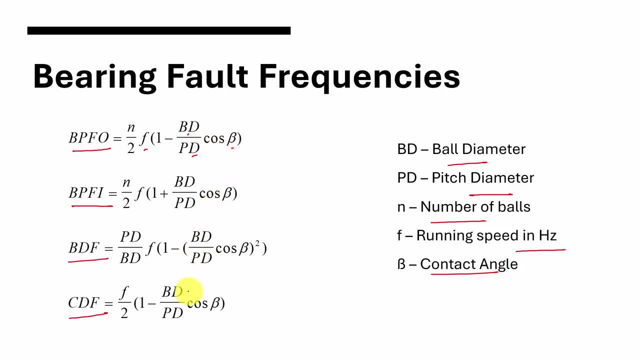 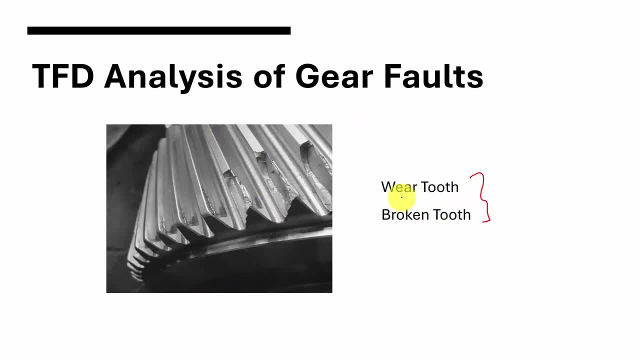 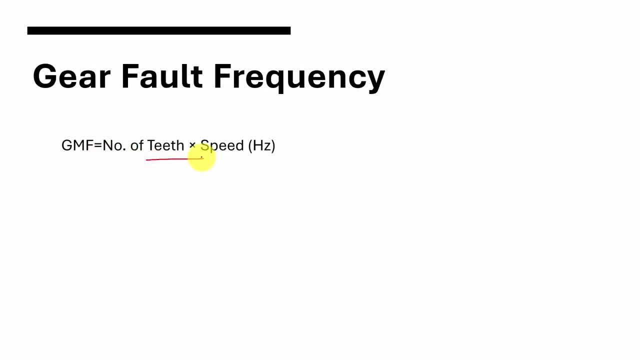 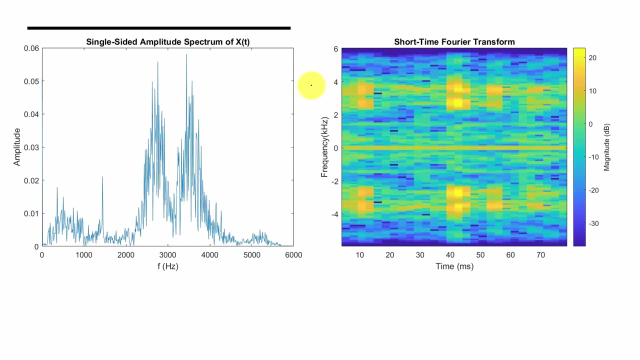 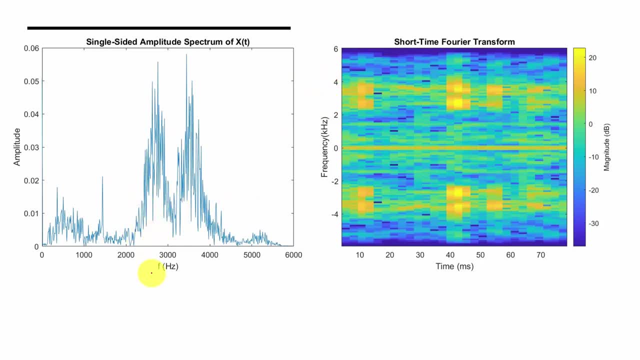 domain analysis of a signal. So this is actually the frequency domain signal. So I have used f of t to extract this signal. So here you can see that now I am going to compare the difference between fast Fourier transform and the short time Fourier transform, that is, time frequency domain analysis. 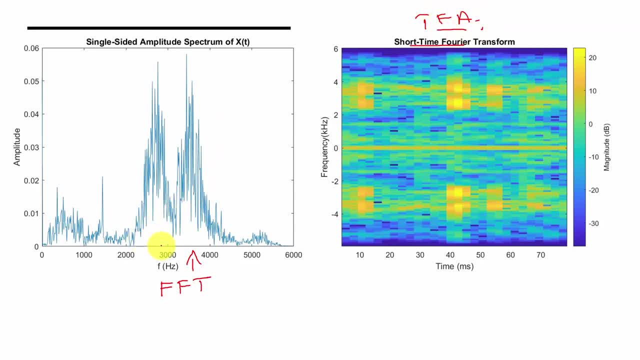 So here you can see that around 2800 hertz. we have a peak and here in the time frequency domain analysis around 2800 hertz. so this is actually in kilohertz. you can see a energy concentration Similarly around 3500 hertz. there is a peak in the frequency domain and here also around 3500. 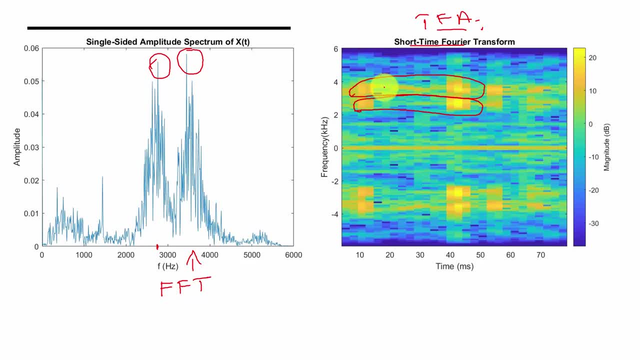 you have a energy concentration. So the fault identification. Now we have the fault frequencies of bearings and gears. So four frequencies for bearing and two frequency for gear, that is, your one for pinion and another one for gear. So in frequency domain analysis we will compare the frequencies of the faults with this. 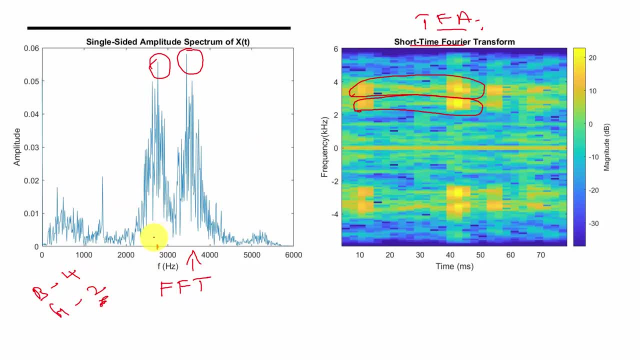 plot. For example, if my gear mesh frequency matches with the peak value in the frequency domain signal, then we can identify The fault is there at the gear. For example, if my BPFO, that is, ball pass frequency, outer race, is around 3500 hertz, then we can confirm that in the 3500 hertz there is a peak which. 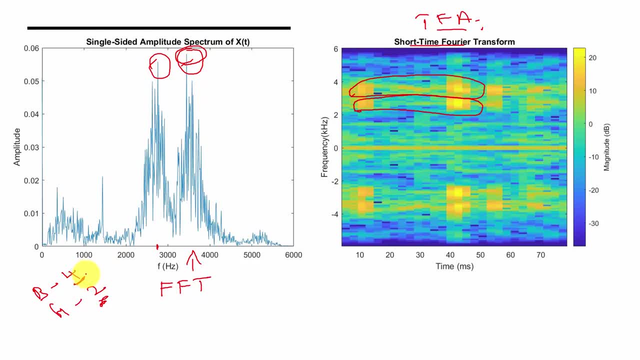 means that there is a fault in the outer race because the BPFO matches with this peak value. So this is the common procedure we are following to identify the faults in the frequency domain. The same procedure you can follow it for time: frequency domain analysis. So here the peak. 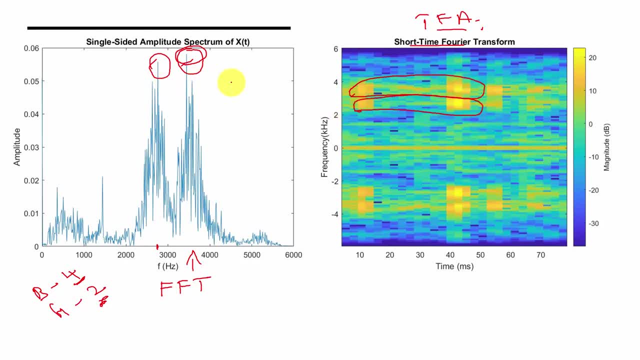 the energy concentration occurs at the place of the peak frequency. So the advantage of time frequency domain analysis is you will have energy concentration at the fault frequency or otherwise. it needs harmonics. Harmonics means may be you can have it at 1-X or 2-X or 3-X. 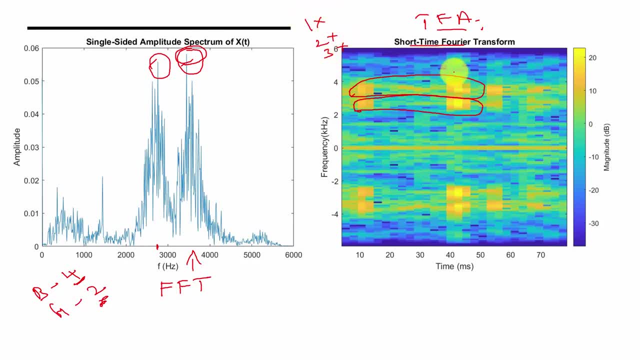 So this is how we can identify the faults in the time frequency domain analysis. Now you may ask that then what is the advantage ofικ I? this is the question. they used two albumin revolutions to compare the faults from the peak. whenever the tempo is placed on peak nominal values also, and these often do it this way- 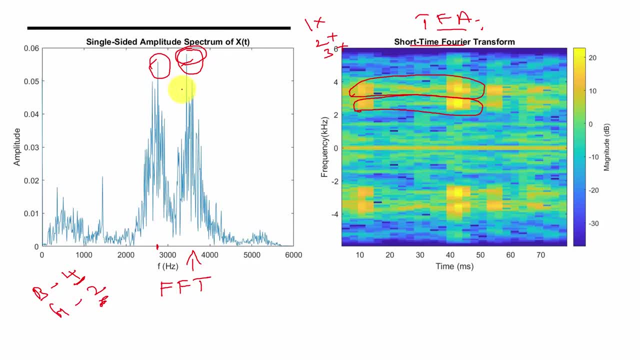 time frequency domain analysis over frequency domain analysis. so actually this is a basic transform. short time. Fourier transform is a basic transform. now we have plenty of transforms for noise reduction. so here you can see that there are plenty of unwanted noises are there in frequency domain. also. you can see that by using some advanced transforms like CWT. 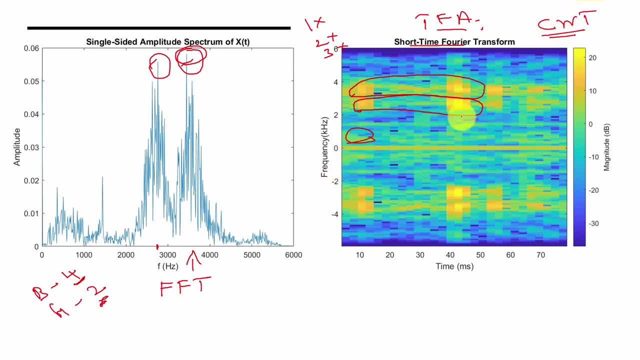 then you can neglect these unwanted noises and the cross terms so that you will get an exact energy concentration at the fault frequency. so you will not have these unwanted noises when you are using the advanced transforms. so that is the advantage of time frequency domain analysis. you have plenty of transforms. so based on your need and your application, you can select the. 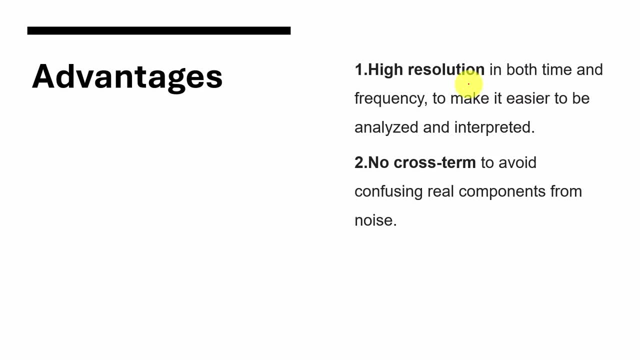 transforms accordingly and you can identify the faults. so these are all the two major advantages, as you see here, said earlier, it has high resolution in both time and frequency, so you can extract both the time and frequency domain informations from the time frequency domain plot and there is no cross terms. 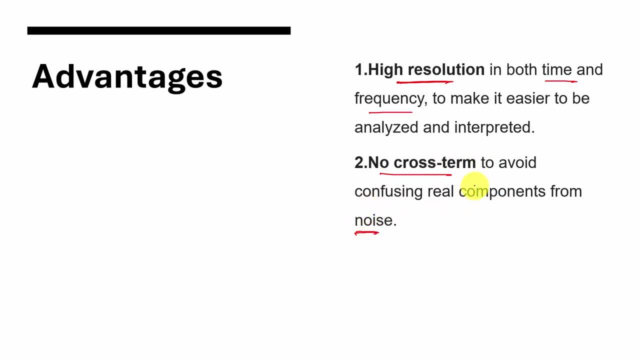 so cross terms means it avoids the unwanted noises, because when you are performing a time frequency domain analysis with the help of any advanced transforms, then you can remove the unwanted cross terms so that the fault identification will be effective. so this is a time frequency domain analysis of vibration signal, now the methodology of fault identification, for example, 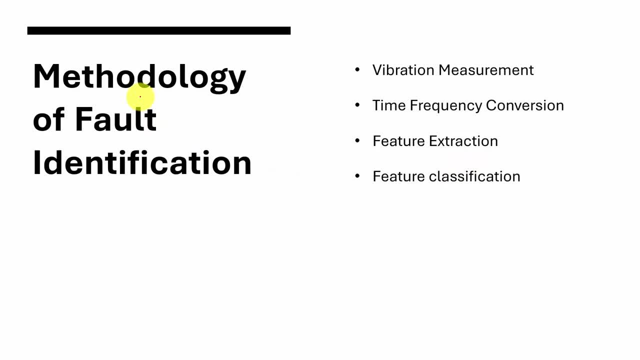 if you are installing a system for continuous monitoring that is, 24 bar 7, you are going to monitor the system means then you need to prepare a methodology for fault identification. okay, so this is the methodology when you are using time frequency domain analysis. so initially we are: 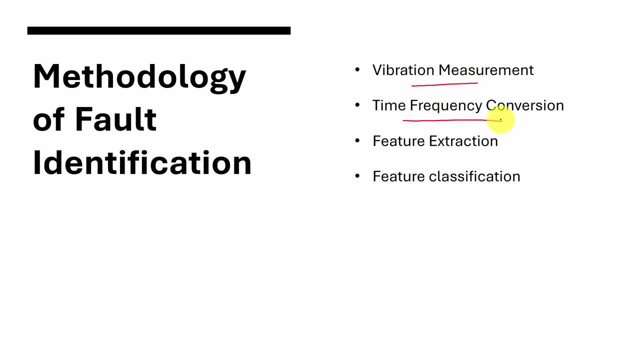 going to measure the vibration signals, then we are going to convert the vibration signals measured into time frequency domain signals. so you can use any one of the transforms: either you can use FSTFT, or you can use wavelet transform, or you can use CWT, or you can use any one of the transform to convert the time. 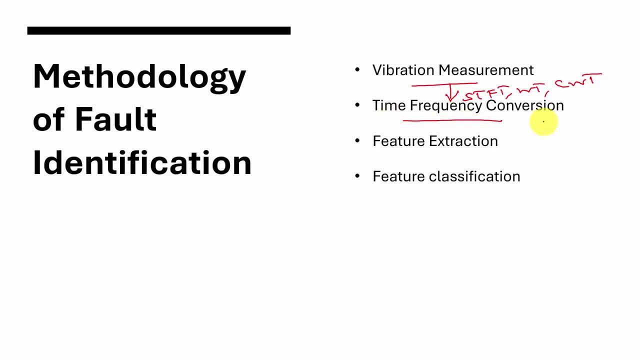 domain signal into time frequency domain signal. so now we have a time frequency domain image, but with this image you cannot conclude that the fault occurs in a particular system, which means that you cannot directly conclude by visualizing the images. so what do you do? what researchers are following is: they are extracting features. okay, so they are extracting. 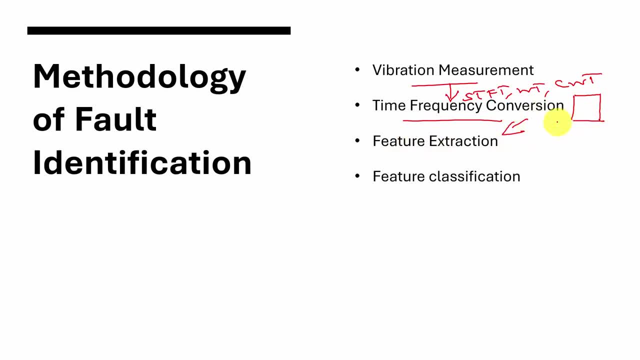 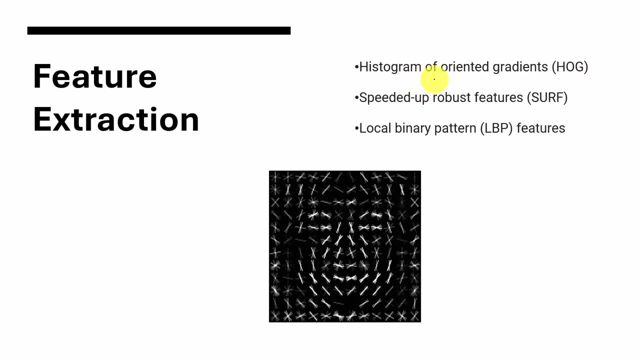 the information about the faults from the time frequency domain signals and from the extracted features. they are going for future classification. okay so in general. so these three are used by researchers in future extraction. okay so. they have used HOG histogram of oriented gradients and some of them have used speeded up robust features and LBF features. okay so. 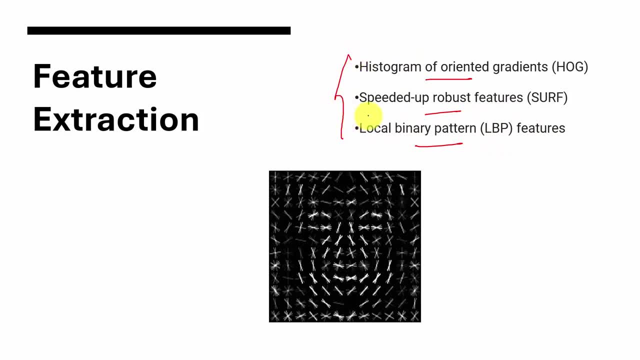 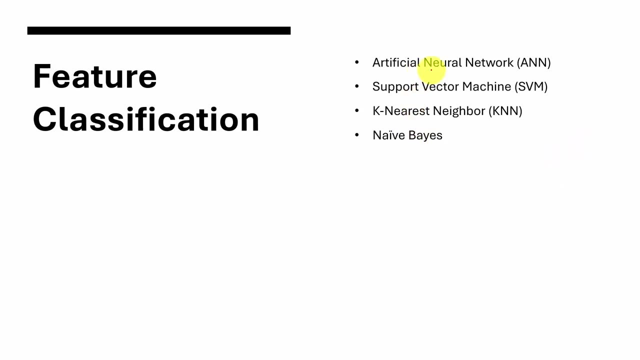 So these are all the commonly used future extraction technique for time frequency domain images. So you can use any image future extraction technique for extracting the information from the time frequency domain. So after extracting these features, then we can go for future classification. So for future classification you can use any one of the machine learning algorithm. 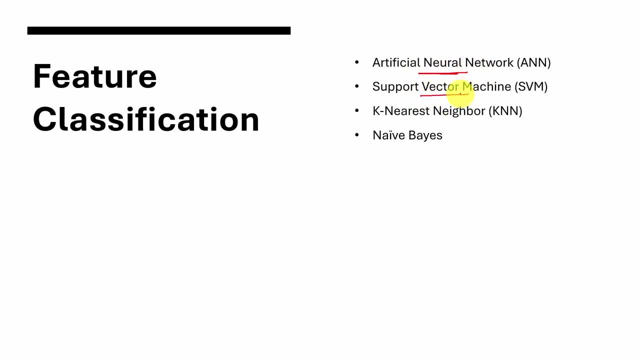 You can use support tractor machine or otherwise. you can use artificial neural network. Then you can use k-nearest neighbor and neighbor bias. So among those, SVM is most commonly used in fault identification with the help of time frequency domain analysis. So here in this methodology we have extracted the features and we have classified the features for fault identification. 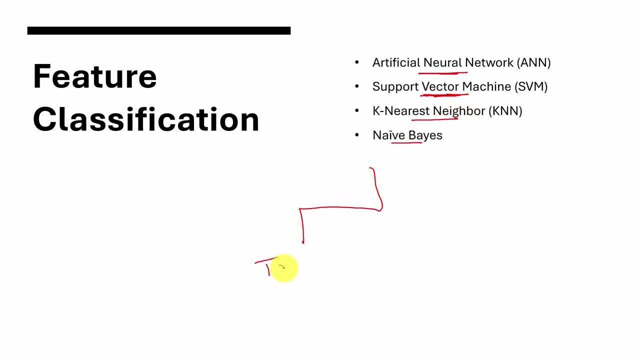 So in this case you need to train your algorithm. So first you need to split your data or otherwise. initially, while installing the machinery, you have to capture the vibration, So you have to create the faults or you have to Induce the faults manually and you have to capture the vibration signals of the faulty system. 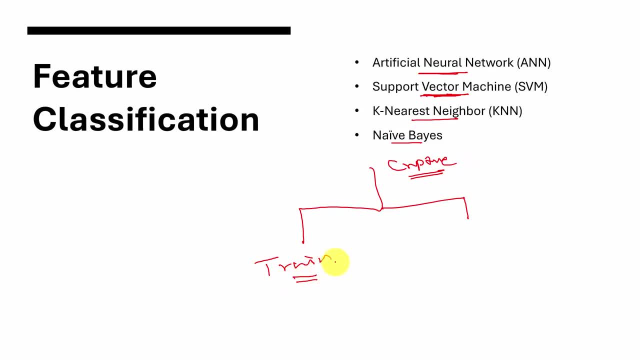 So you have to use that vibration signals to train your algorithm. So these are all the algorithm. So you have to train your algorithm using the captured features. Then, to ensure the effectiveness of your algorithm, then you can test it. So once if you test and if you confirm that your algorithm is working perfectly, then you can go for real fault identification. 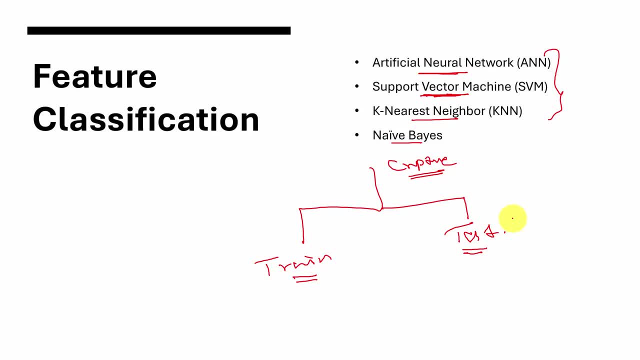 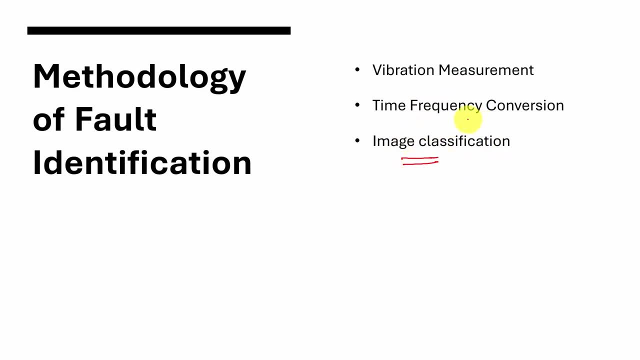 But using the same methodology you can Follow the fault identification. The 2nd advancement is the image classification. So here we are not going to extract the features from the time frequency domain signals, We are directly going to classify the images. So initial stages, vibration measurement. 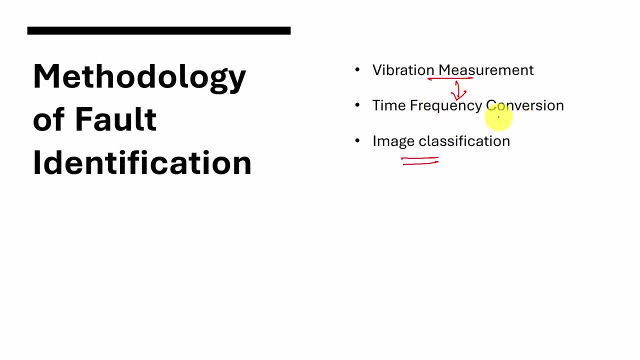 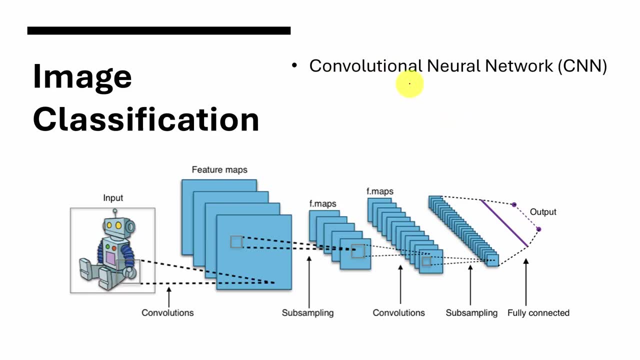 Then time frequency conversion. Then these time frequency images are directly given as a input to image classification algorithm. So in image classification algorithm is most commonly used, but nowadays people are using LSTM networks. Anyway, it's an advancement of CNN, so you can use any one of the image classification algorithm for fault identification. 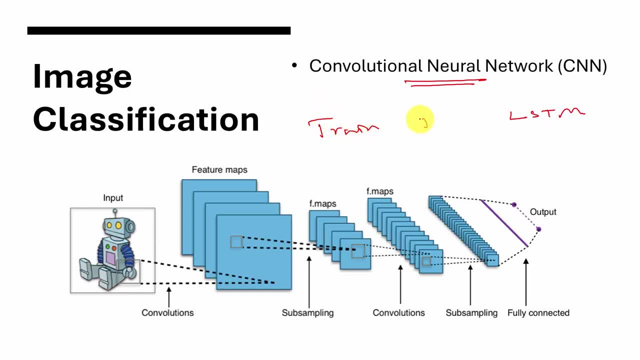 So here also, we are going to split the data into training and test. So here also you need trained data, because without training data you cannot form a methodology like this. You need trained data so that you can confirm your effectiveness of your algorithm. So here,